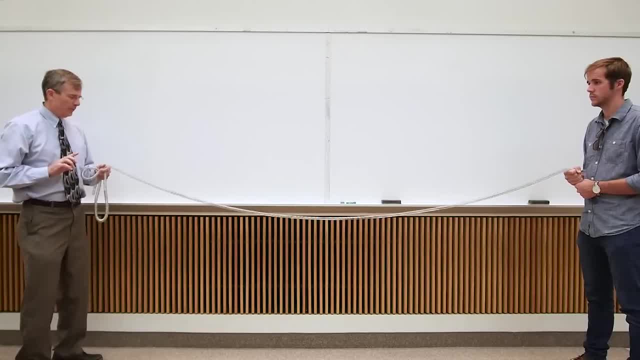 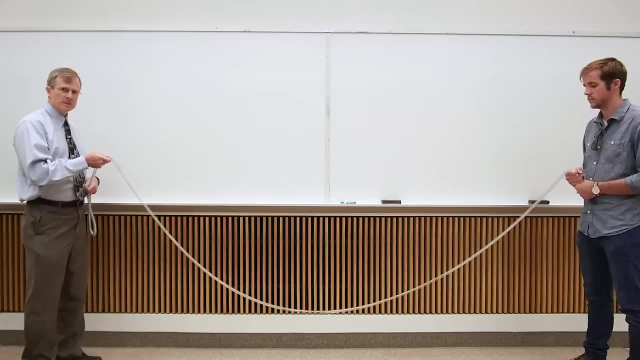 in such a way that the waves created from my side of the string and bouncing off of Parker's coincide with each other and reinforce each other to create a standing wave pattern. So the lowest frequency standing wave pattern is this one. It's called mode M-O-D-E-1,. 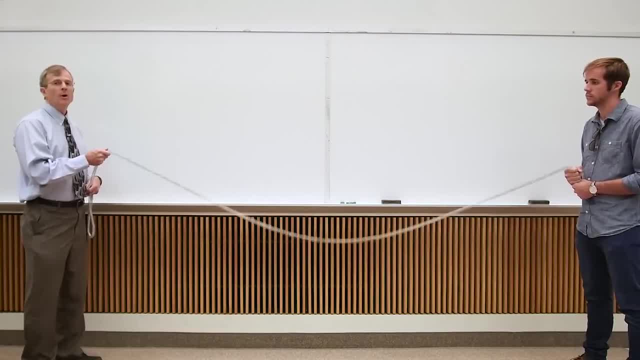 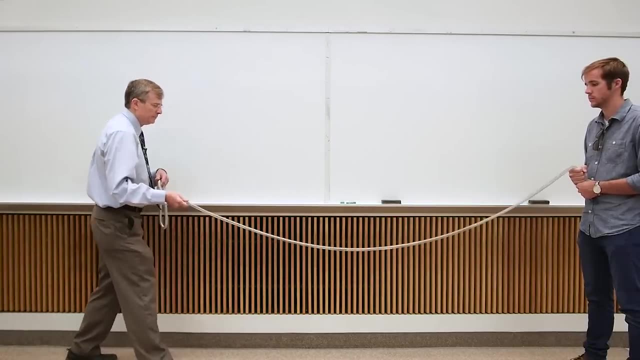 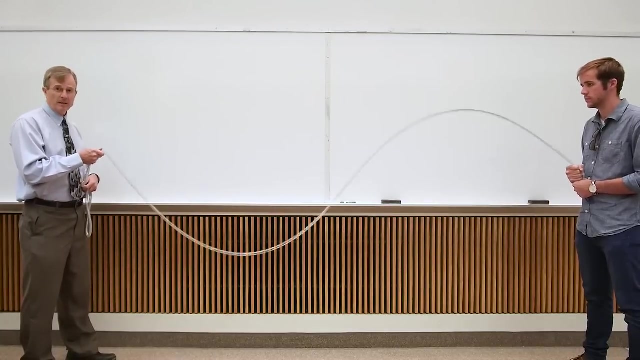 or the first harmonic, or in other words also called the fundamental mode. It's the lowest frequency mode that you can get in a transverse standing wave. If I double the frequency of that mode I get the second harmonic or second mode, and sometimes called the first overtone. 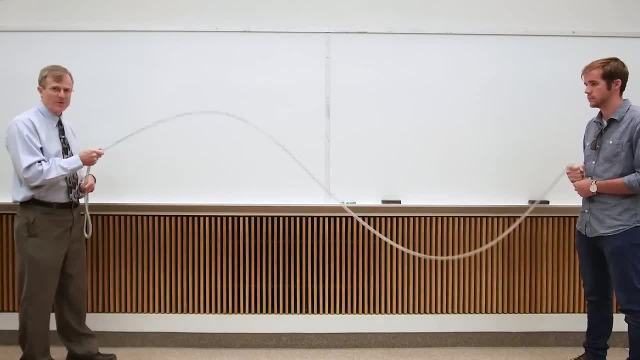 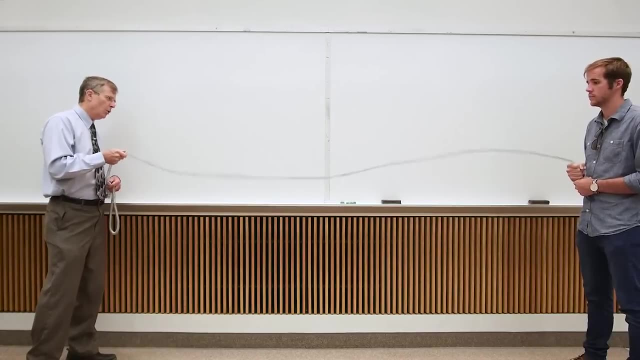 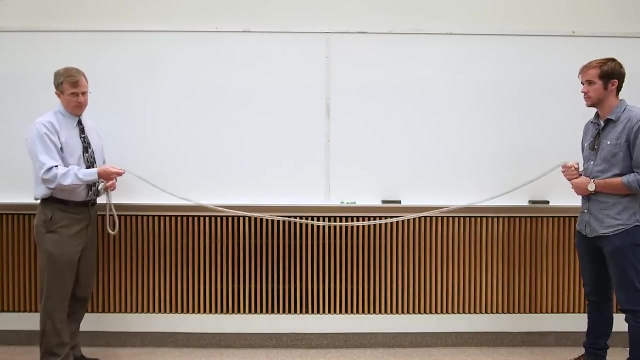 And this one, if you'll notice, is going twice as fast as the fundamental mode. It has a node that's exactly halfway between Parker and me, and that's a node where there's approximately no motion going on. Let's see. So now I'm gonna try and triple the frequency and get a standing wave pattern that coincides with the third harmonic or second overtone. 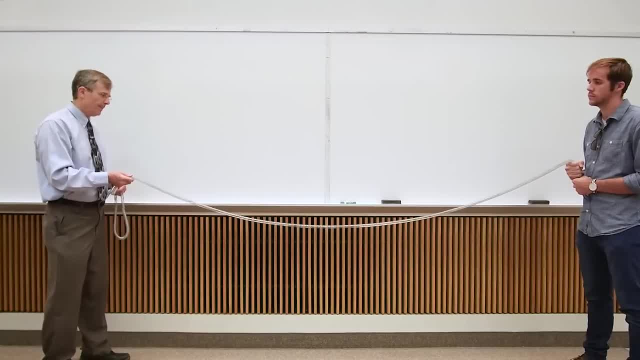 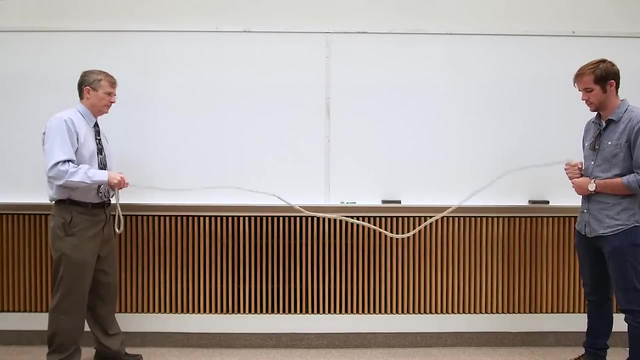 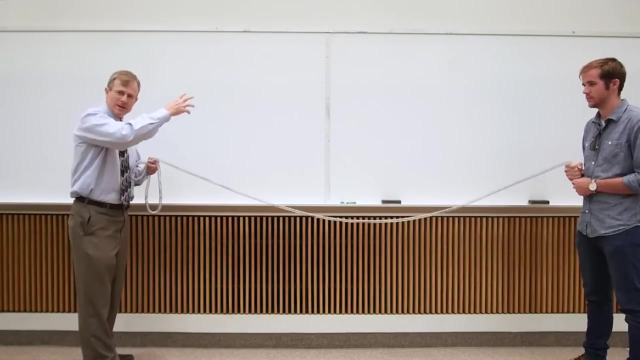 Let me try again. Okay, I think I've got it approximately now. I Think I had it for a little while there. That's the third mode, where the Where the string vibrates in three separate segments. there's actually an infinite number of these modes that you can get, and 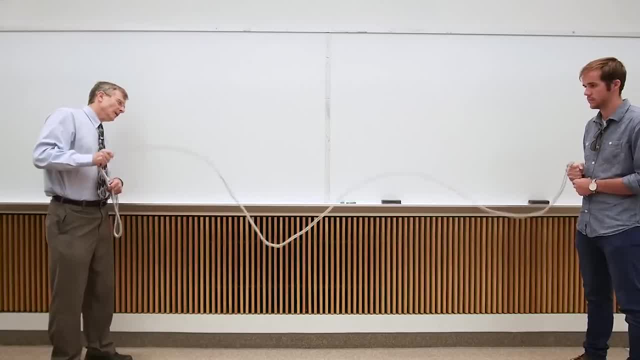 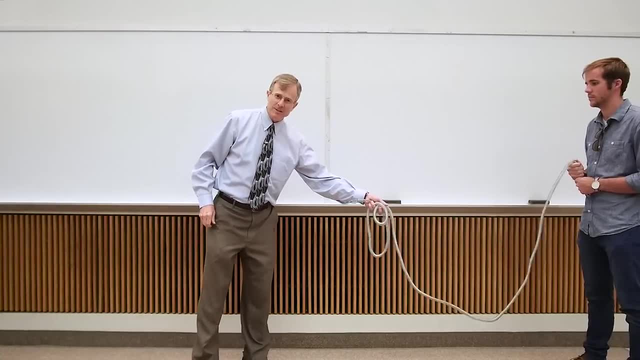 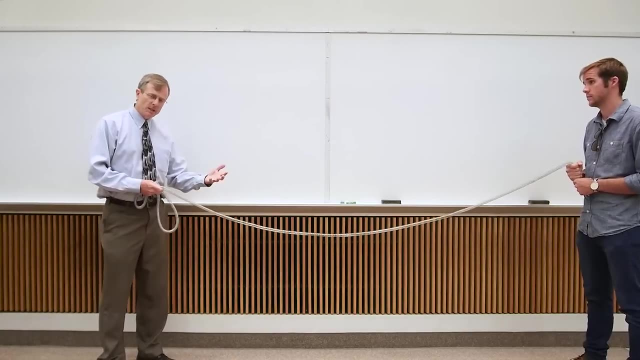 see if I can get one of the higher modes. I think that's four- and And then, if you're really really good, you get five, six, seven, eight, etc. So notice that with each mode There's a particular frequency that I have to vibrate at in order to create that mode. so one-to-one. 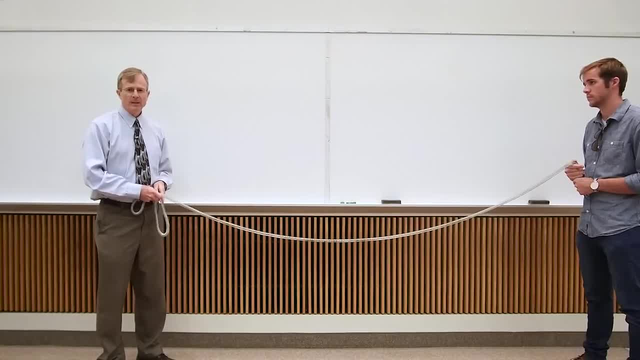 Correspondence between the modes and the frequencies, that's standing waves.